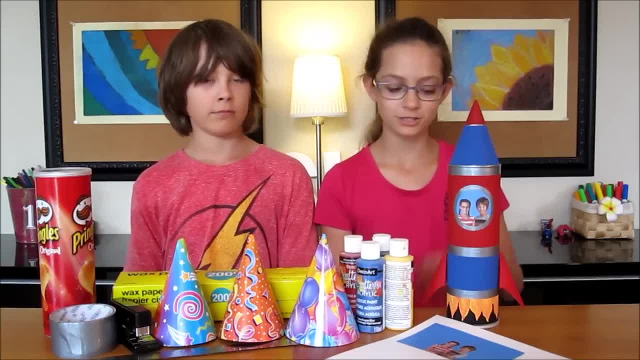 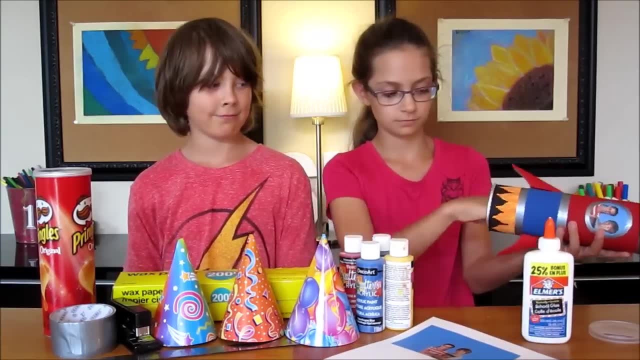 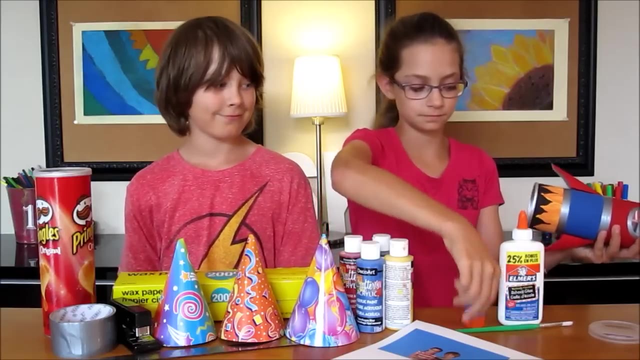 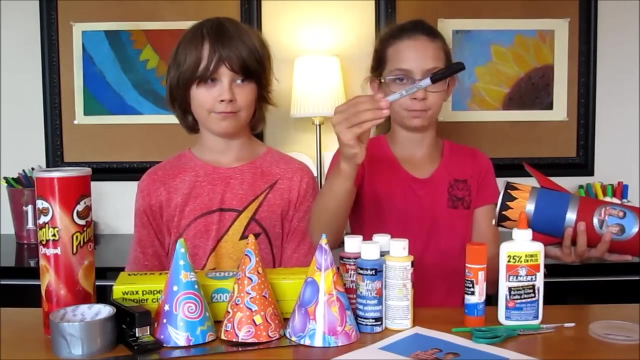 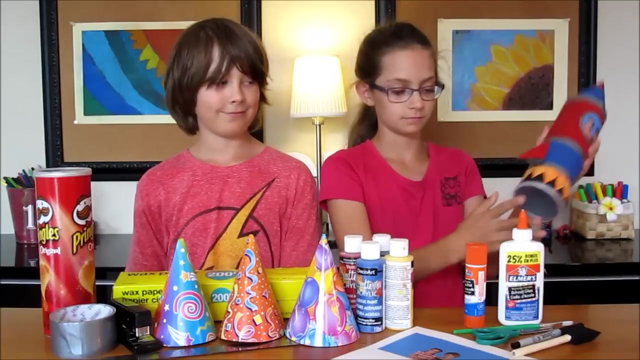 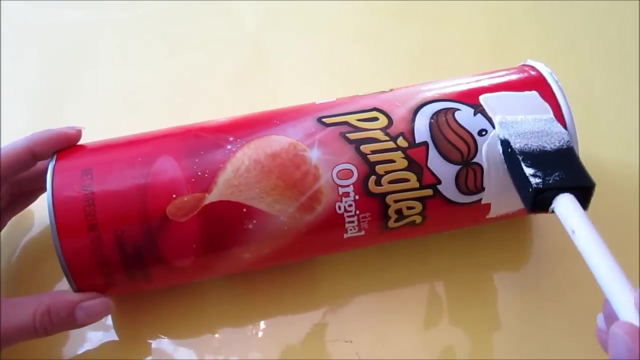 some acrylic. paint a picture. You will also need some glue, a paint brush, some scissors, a sharpie and a foam brush. You will also need tape. Let's start. You will need some glue. You will also need some paper. 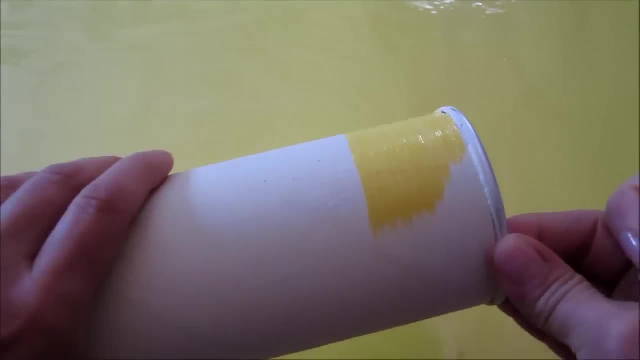 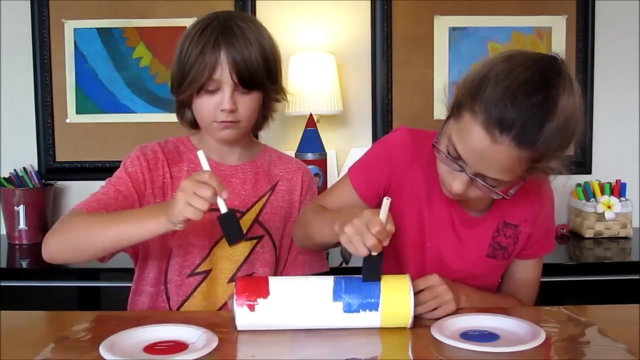 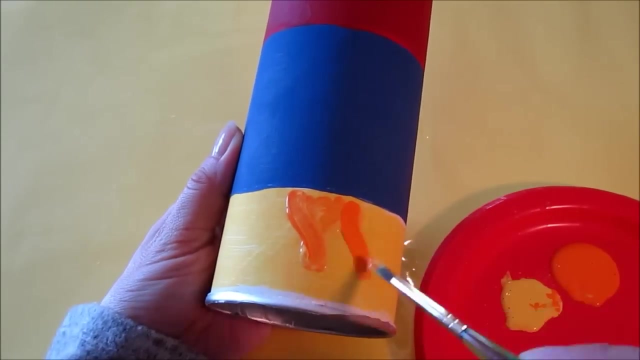 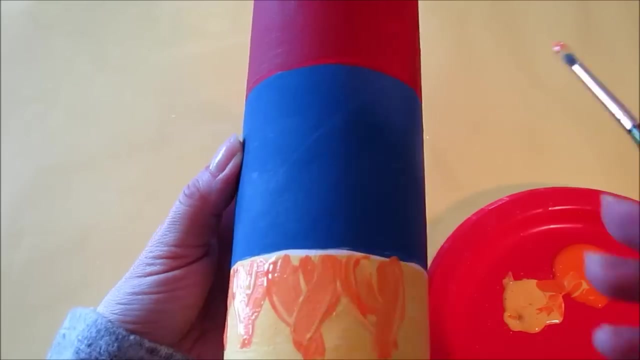 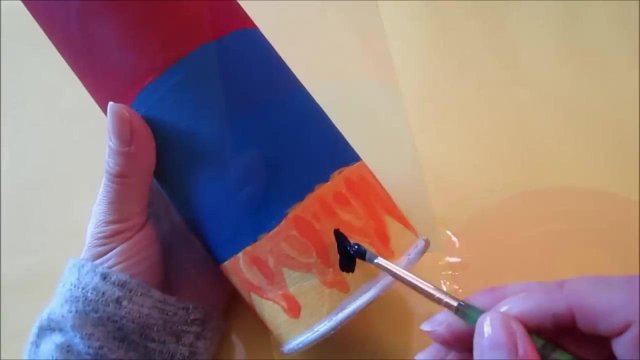 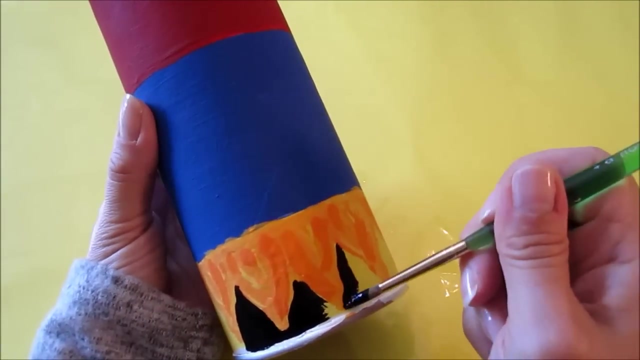 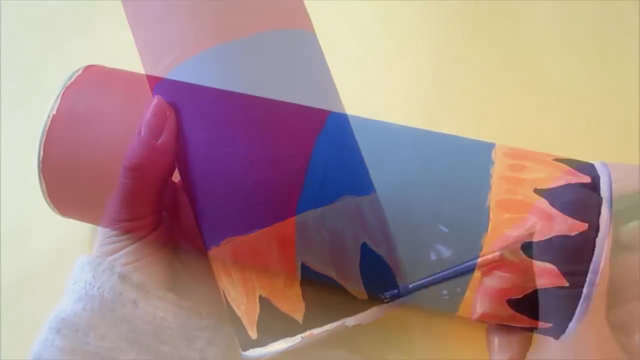 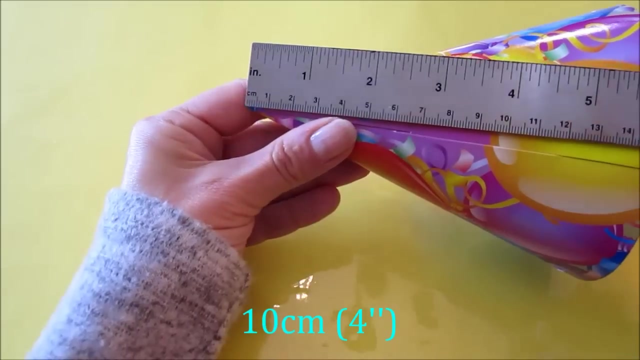 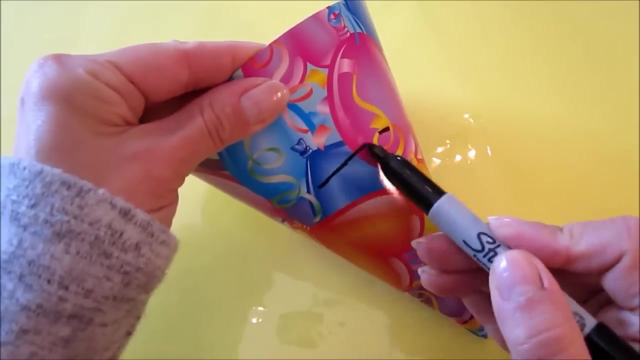 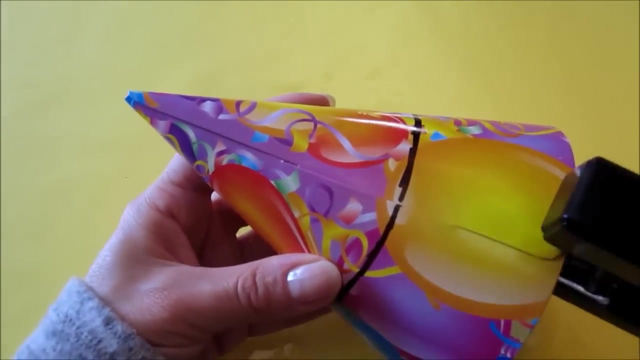 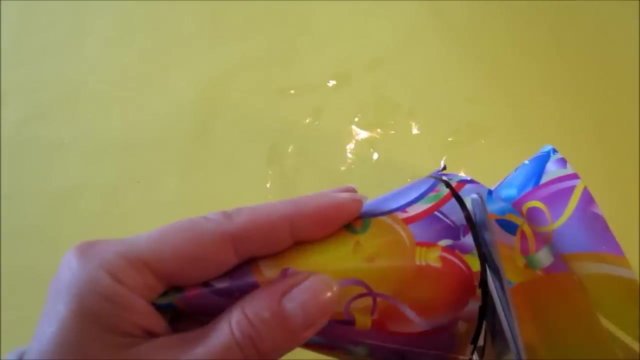 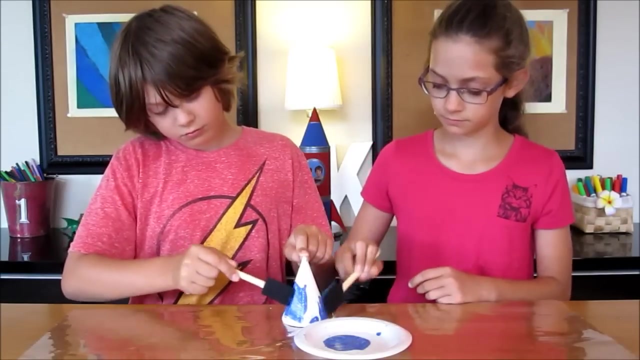 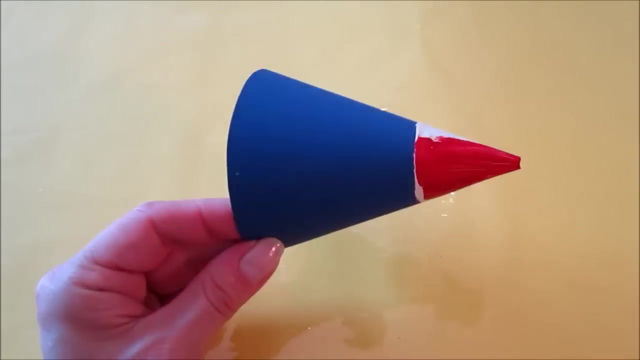 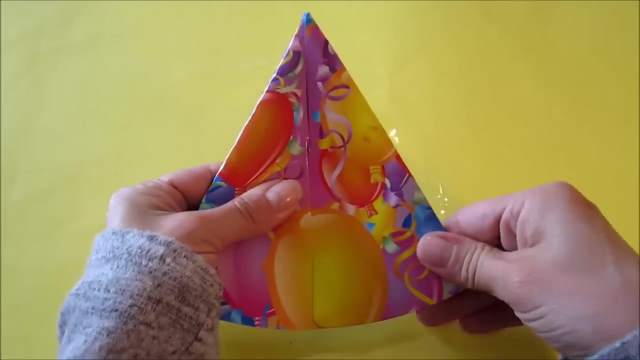 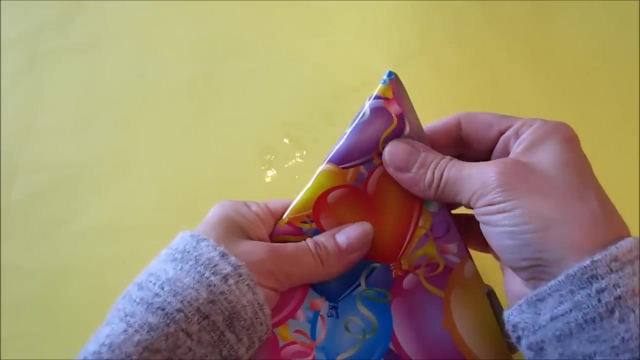 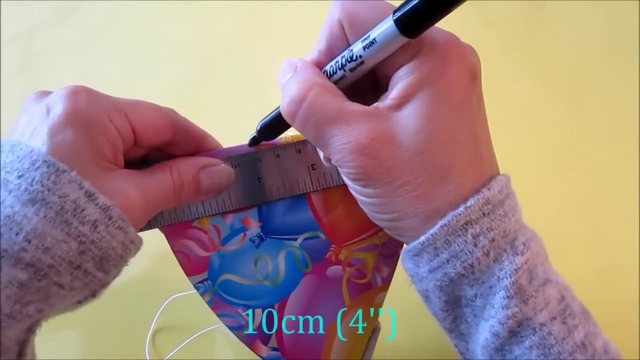 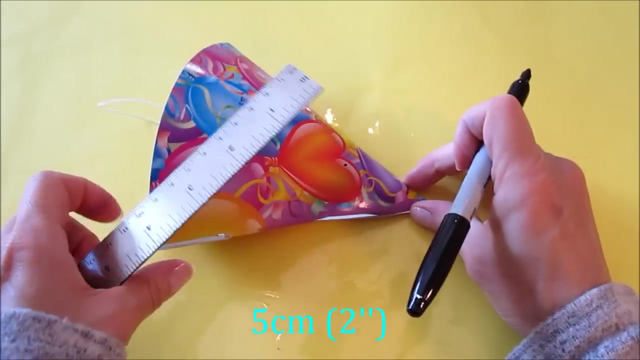 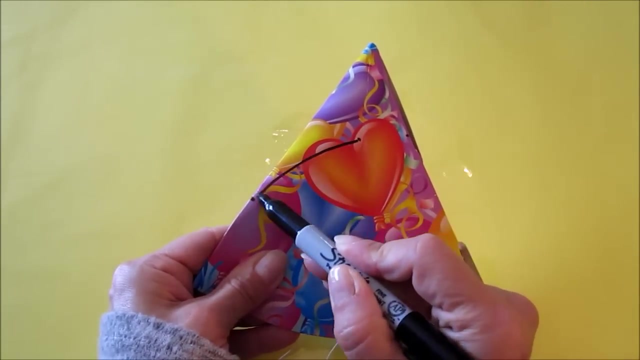 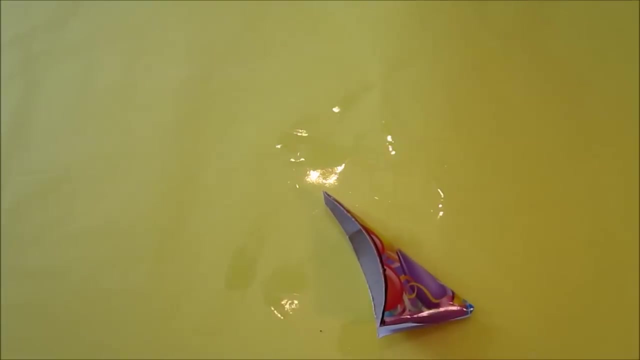 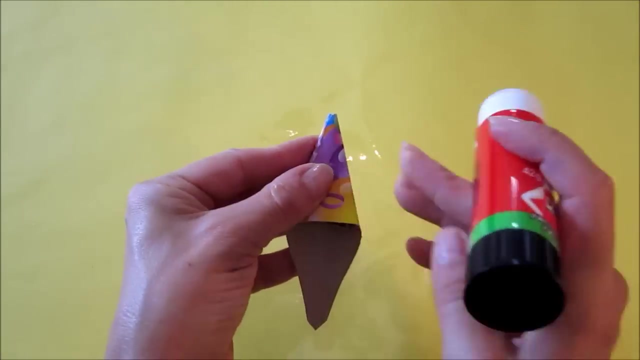 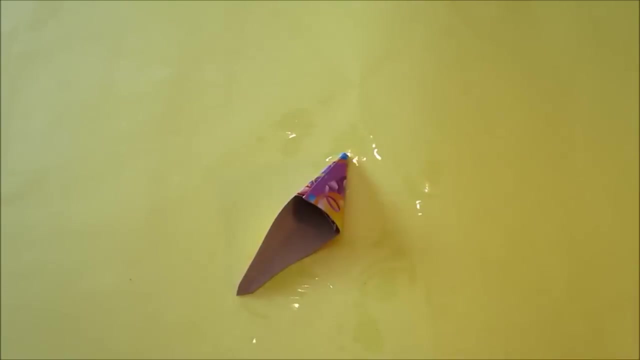 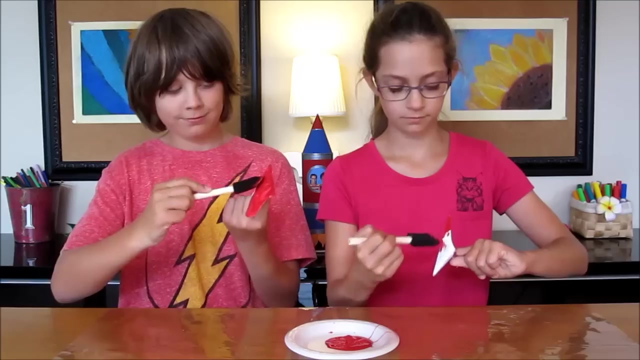 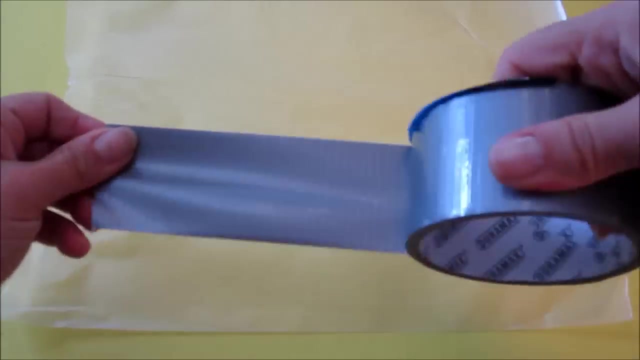 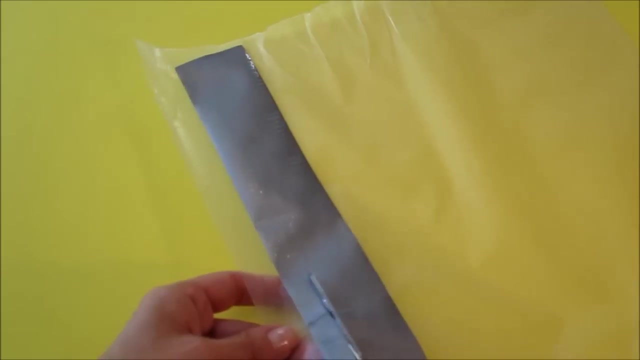 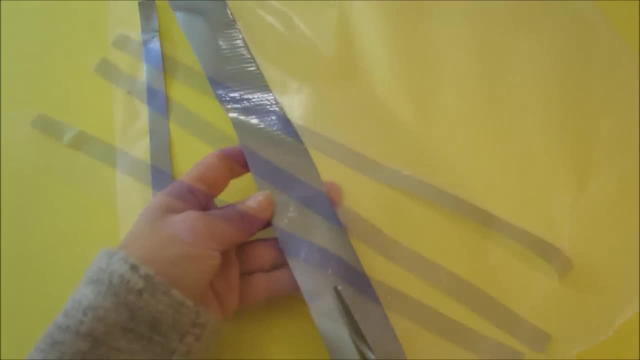 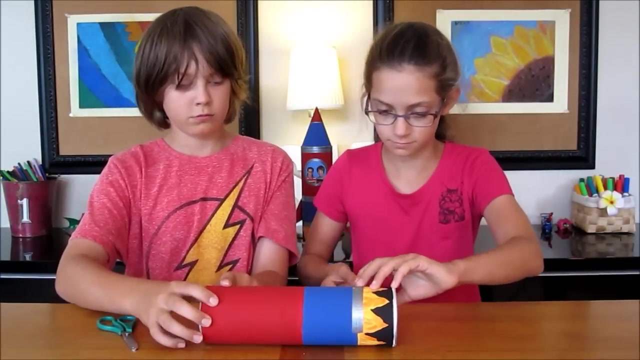 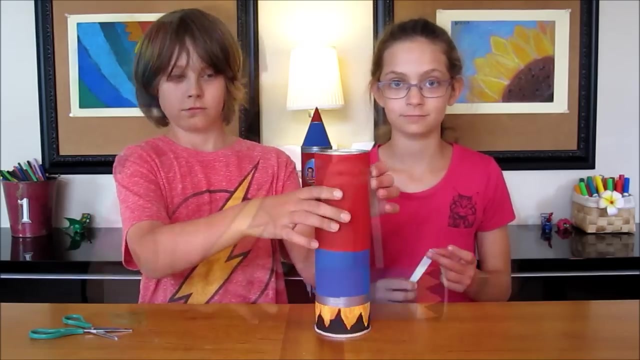 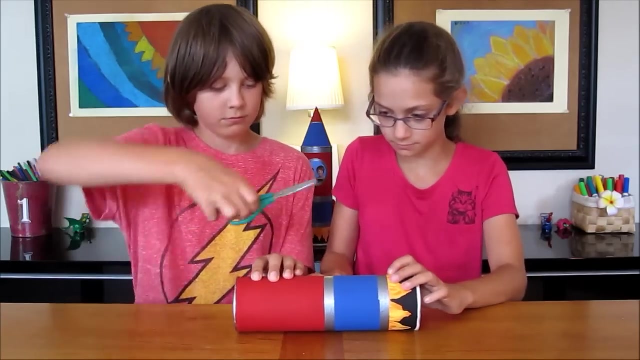 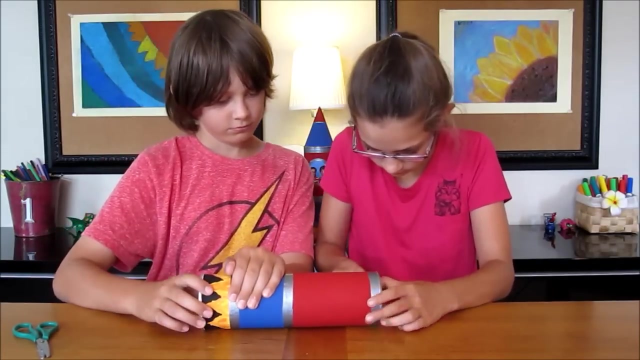 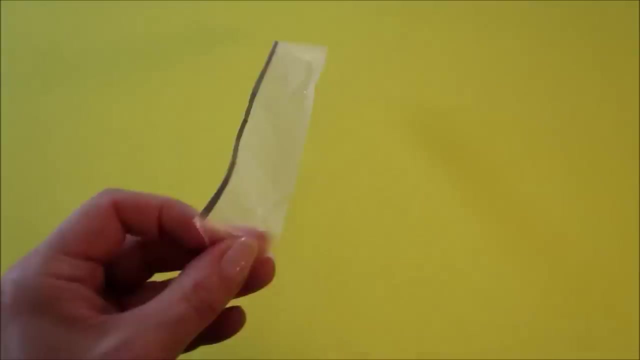 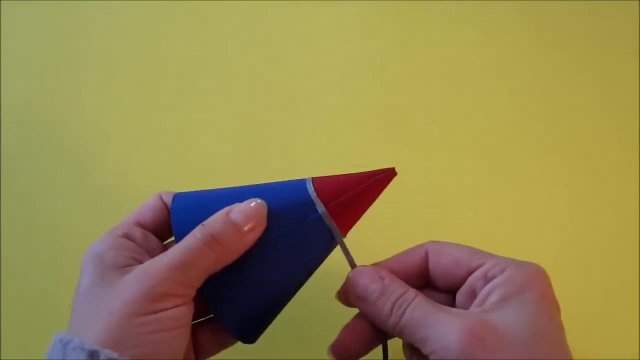 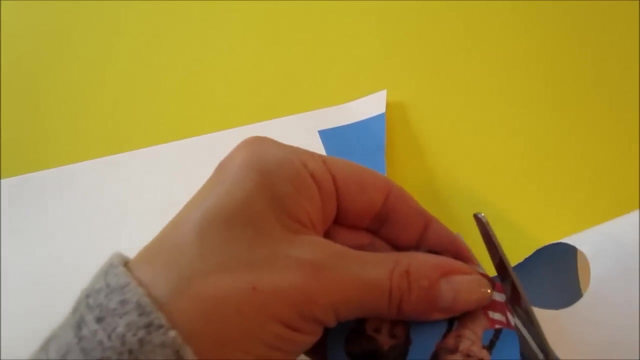 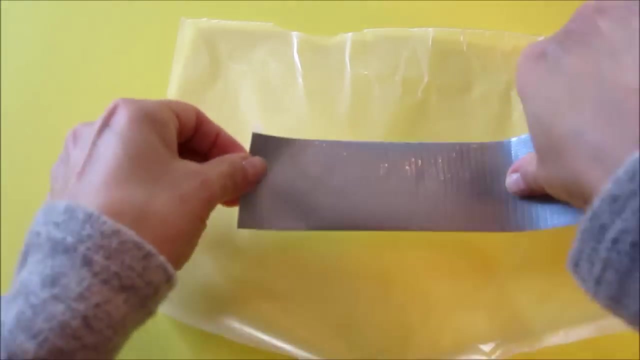 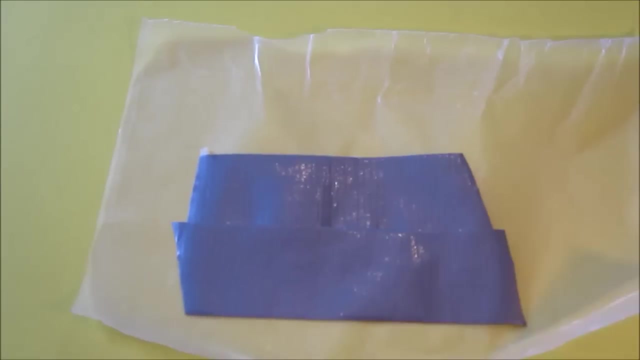 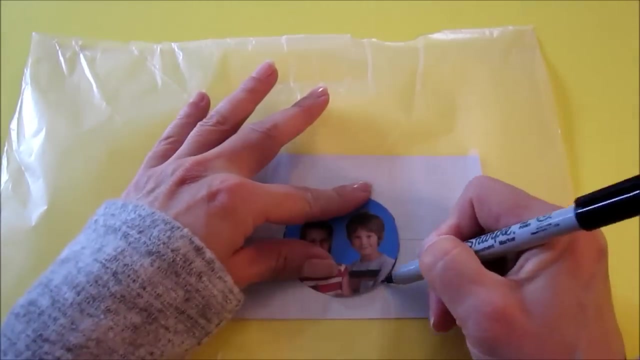 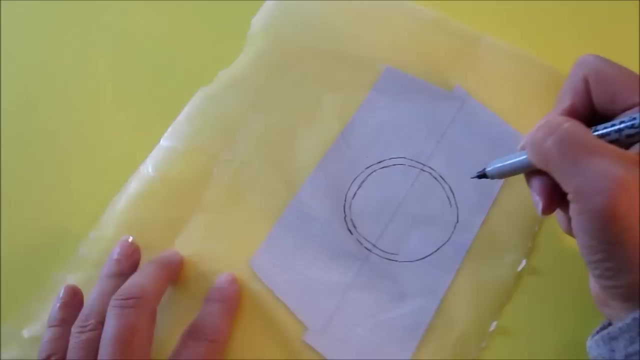 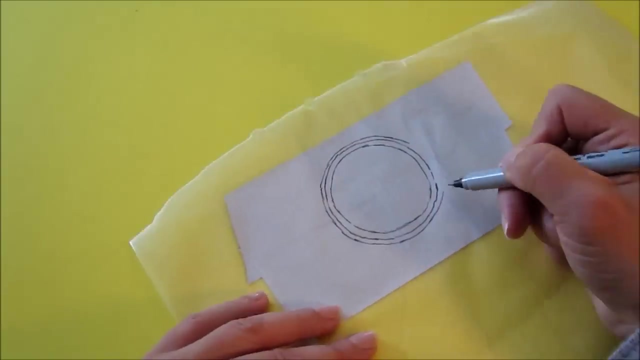 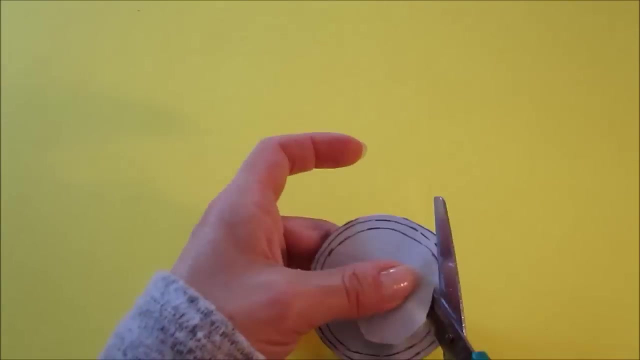 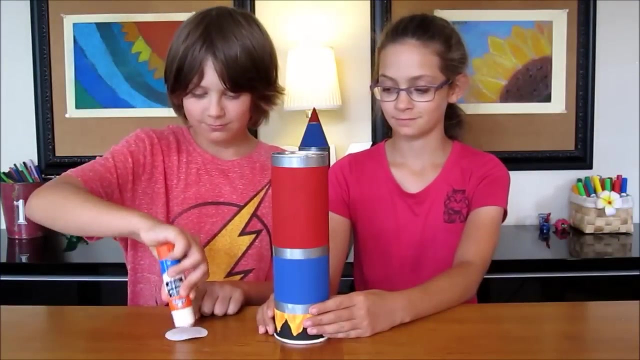 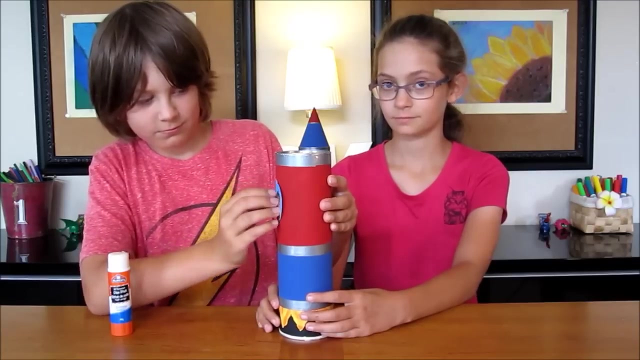 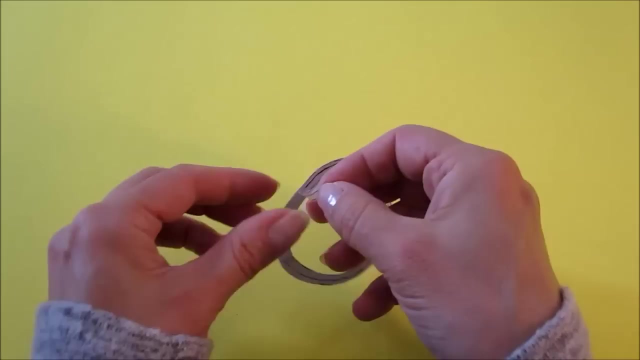 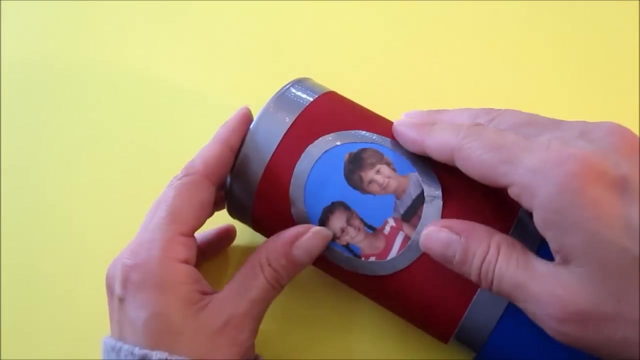 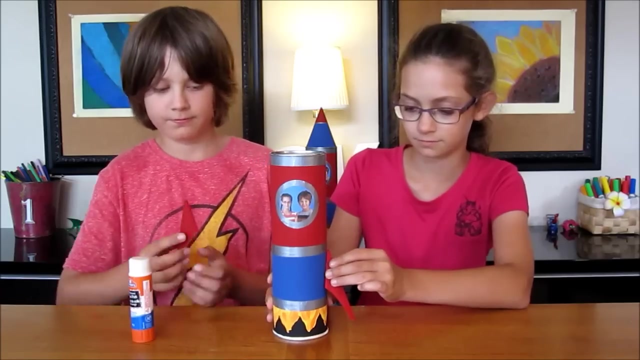 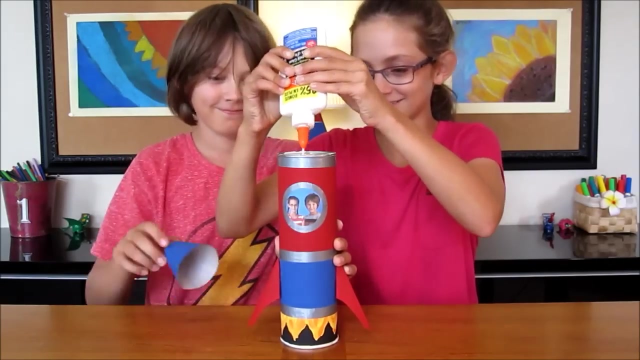 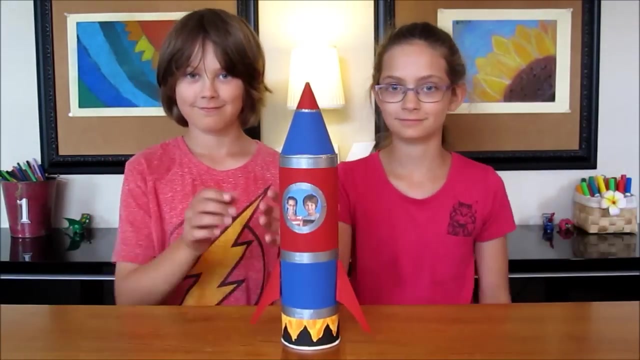 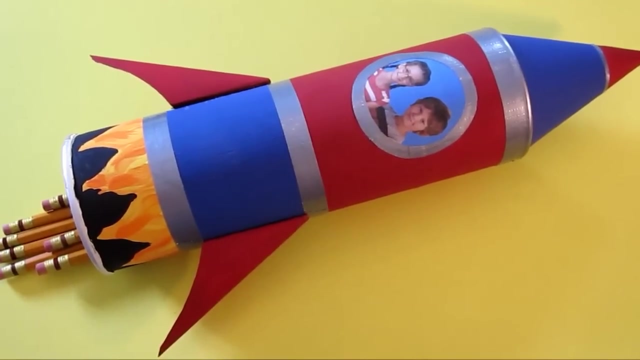 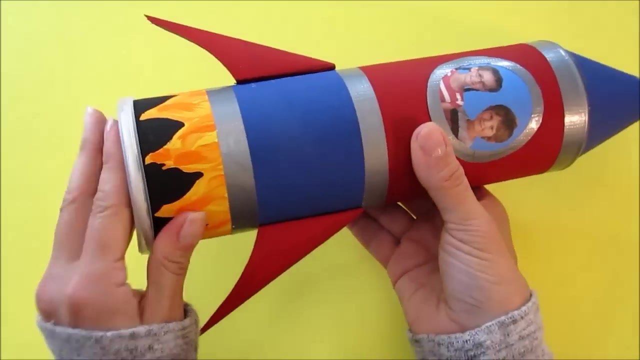 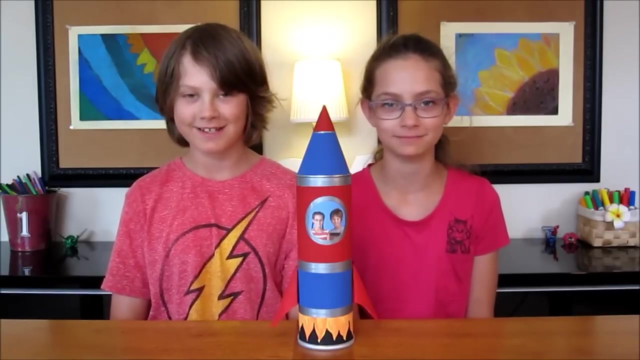 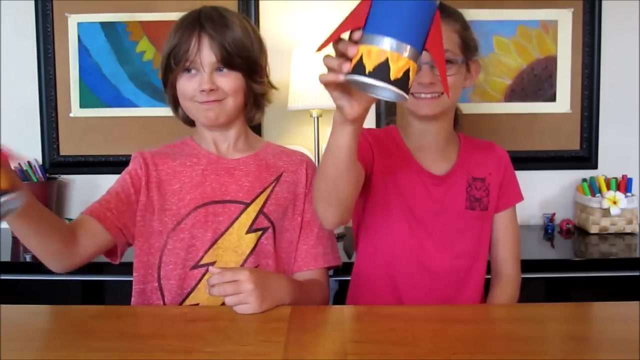 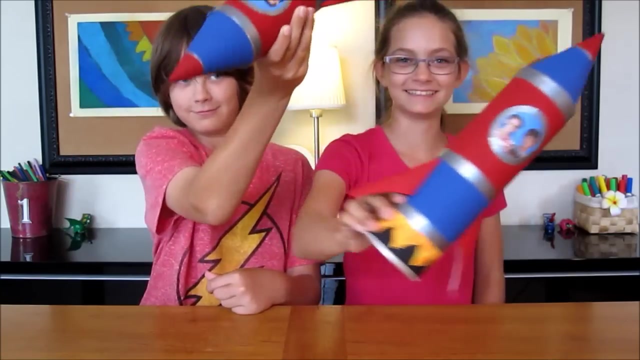 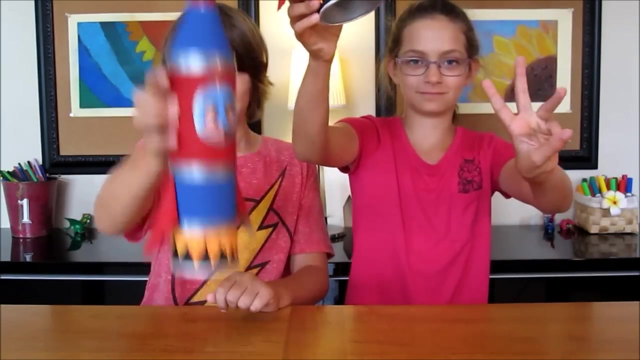 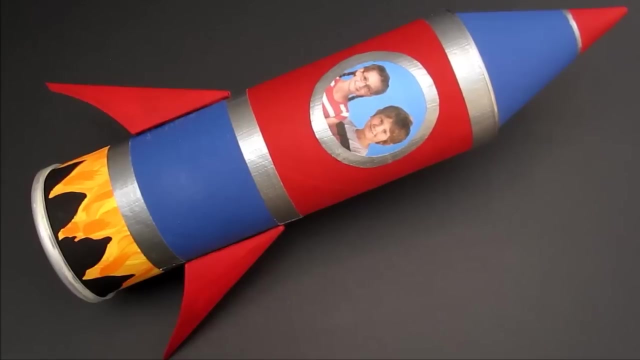 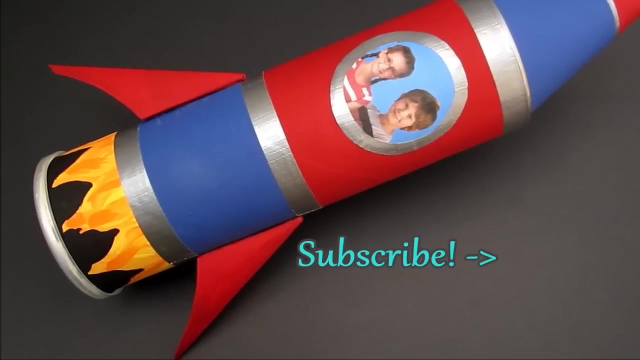 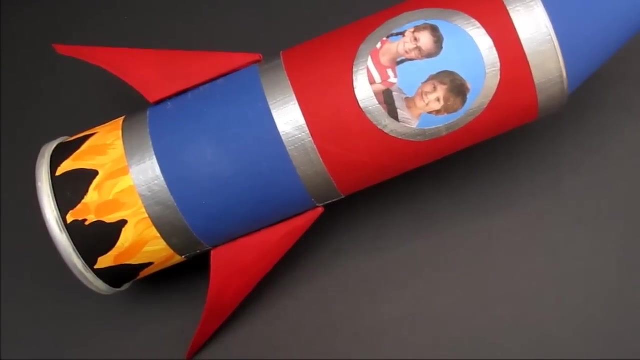